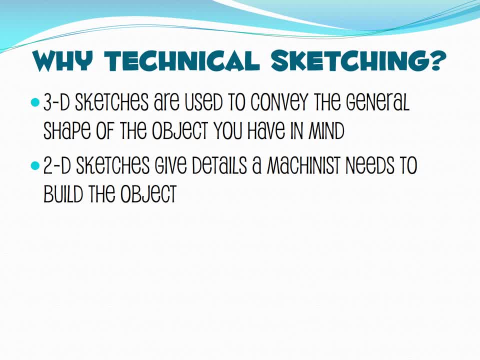 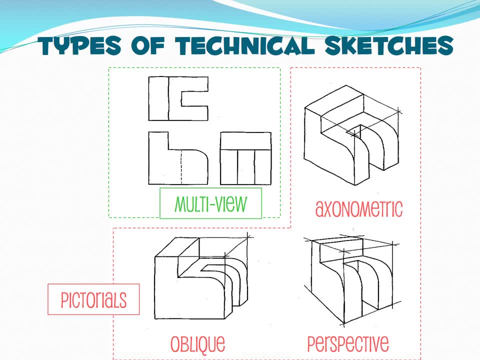 your object be. We'll learn details about all of those things and we'll learn about some specific types of three-dimensional and two-dimensional sketches. For starters, here we have four different types of technical sketches. The multi-view is our only two-dimensional sketch that we'll study. 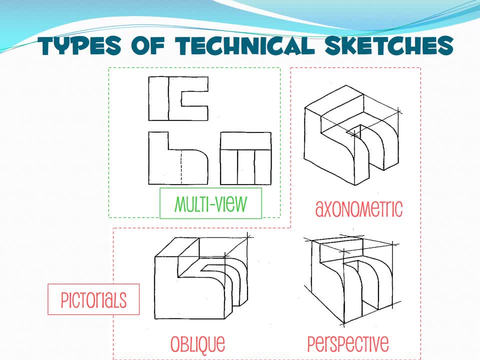 and it shows one side of an object on each view. Pictorials which are three-dimensional ones, show three sides of an object in just one view, and you'll see that there's three different types of pictorials: exonometric, oblique and perspective. Exonometric is most commonly. 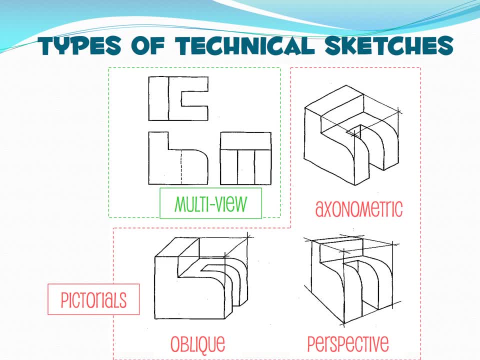 is the most common. I apologize, exonometric is the most common pictorial that we use and a specific type is synonyms of axonometric is called isometric. We'll talk more about that in a moment. That's the one that we're going to focus on, but we also have two other types. 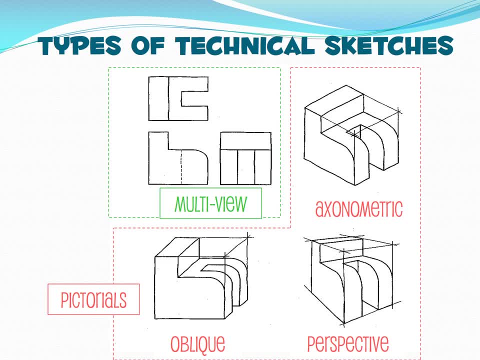 such as oblique and perspective. Architects most commonly use perspective drawings, and perspective drawings are ones in which the top view is minimized. Think about it If you're an architect. typically, we don't care so much about how the top of a building looks, but we 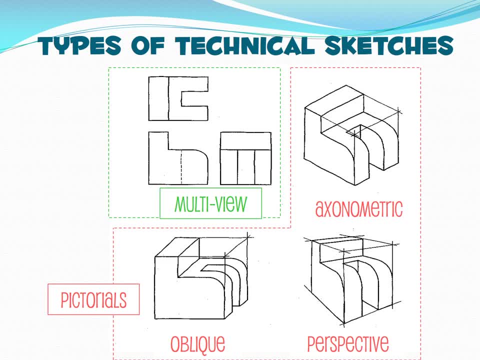 do care about the sides. An oblique drawing, on the other hand, really focuses a lot on one particular side of your drawing, and both the top and the other side are minimized. An example of someone who might use an oblique would be someone who's making cabinets. They really don't care. 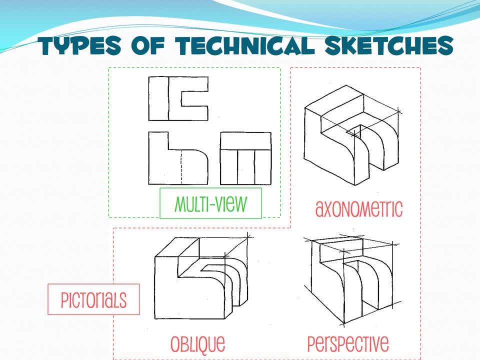 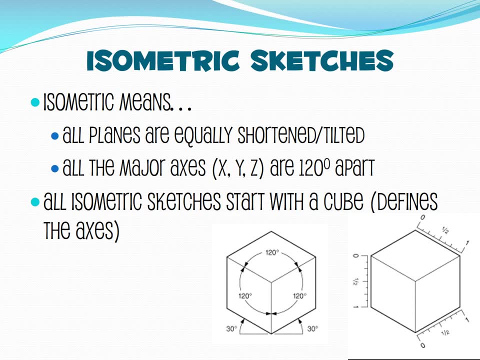 about what the sides and the top look like. They care a lot about the front of the cabinet. Again, the one that we're really going to focus on is an example of axonometric called obliques. We know that that term iso means the same, and so in an isometric sketch, all planes are equally. 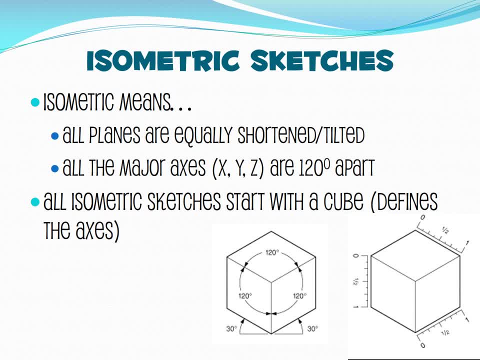 shortened or tilted, and all the major axes, the x, y and z axes, are 120 degrees apart. All isometric sketches start with some sort of a cube- or maybe not exactly a cube, but a rectangular prism, depending on our dimensions, And it's that cube or rectangular prism that defines our axes.